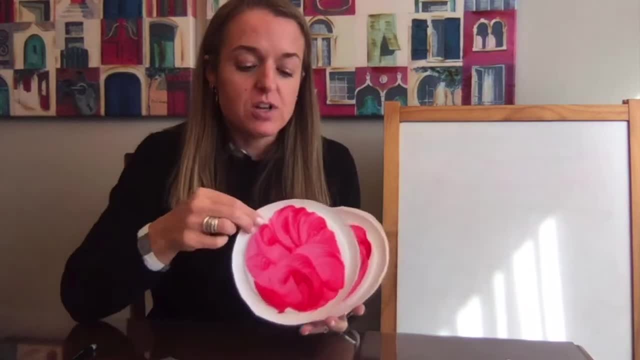 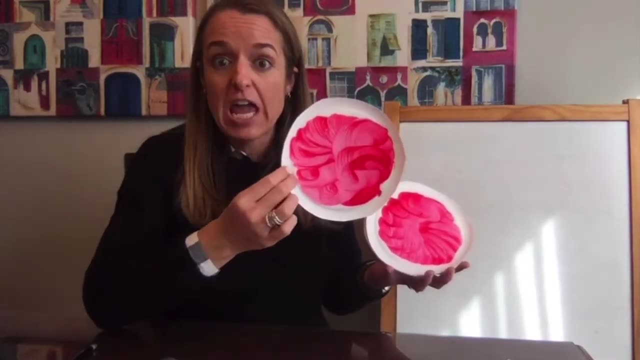 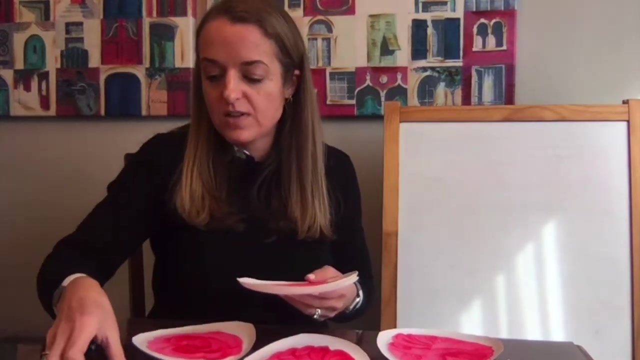 I actually made these three years ago, so I'm reusing them, which is awesome. So this is my thin crust pizza, or my- we're going to just say- regular crust. So it's just one of these. I have one for each kid, So I have eight of these. You give each kid one pizza, And for folks that are: 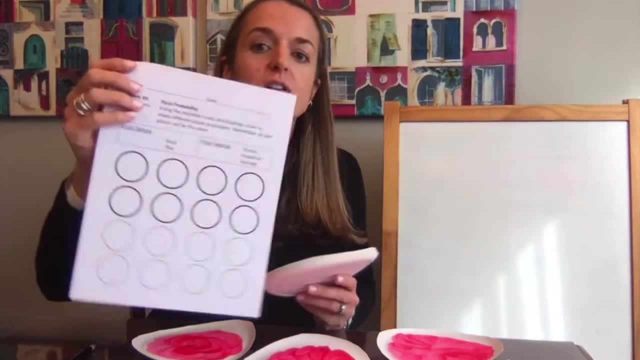 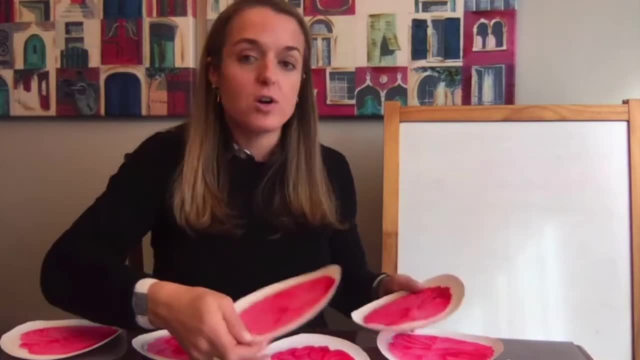 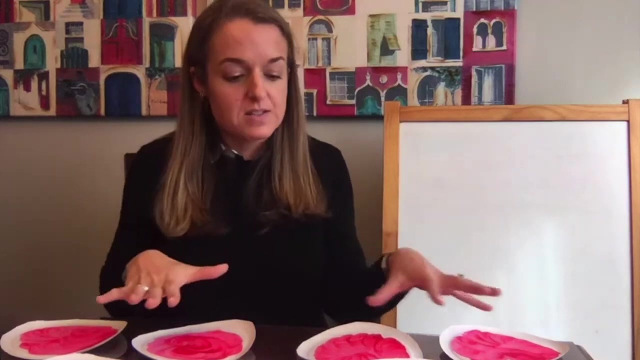 doing it at home. you can just draw circles on a piece of paper to be your pizza and you can draw the same thing that we're doing. Grab some markers, some crayons and you can do the same thing that we're doing- um- just with drawing. So we have eight pizzas to go with our eight um. 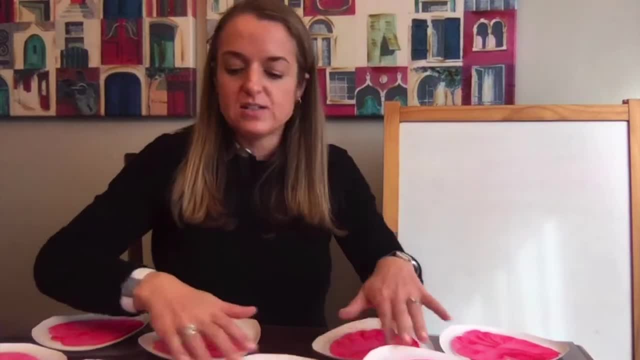 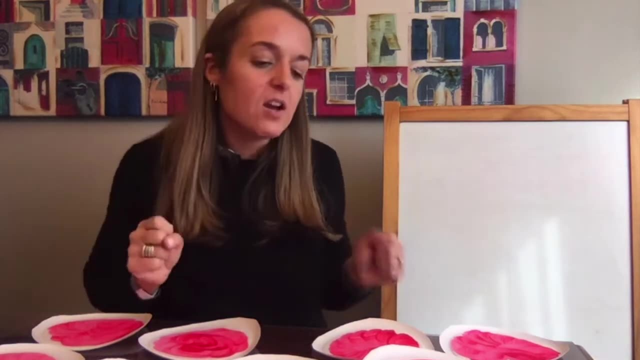 eight students, Okay, So everybody gets eight. Try aim for seven or eight, um, no matter how many kids you have. Okay, So today we're working in a pizza shop and in our pizza shop we have three, three toppings possible. Okay, So all this is everybody's pizza has this. 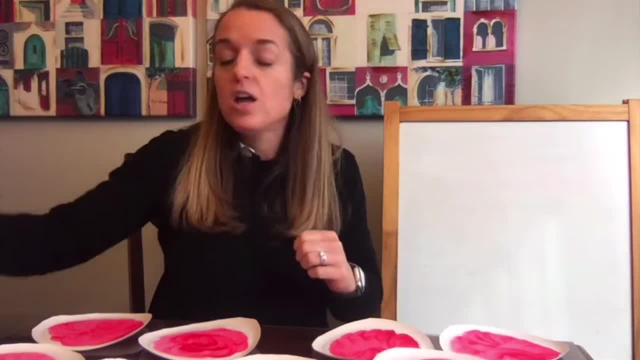 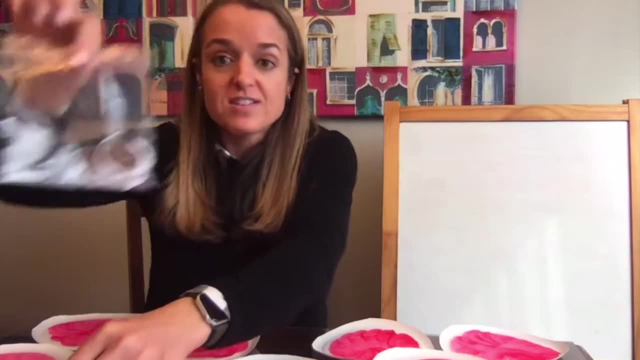 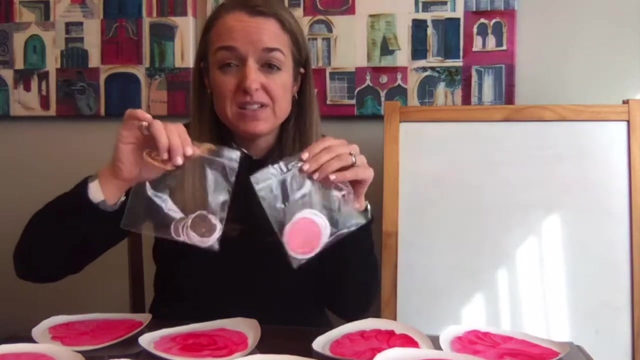 that's sauce, but we're not going to count that as a topping. Our toppings are cheese. Guys, this is shredded paper, just from our home shredder. This is cheese. We have sausage and we have pepperoni And guys for later on, I've got some other toppings. I just Googled pizza toppings online. 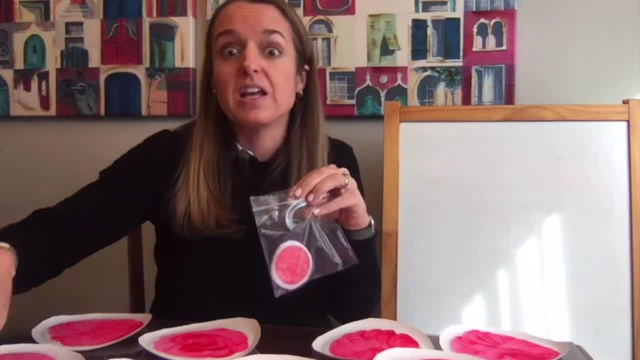 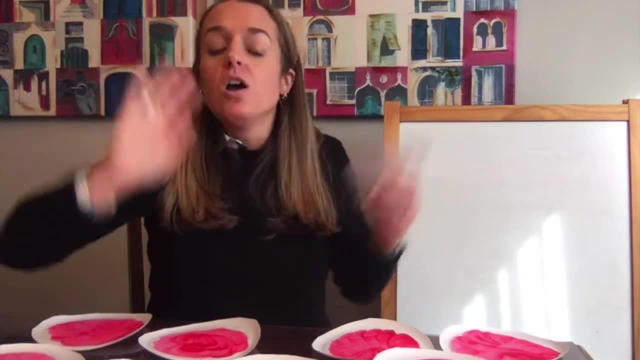 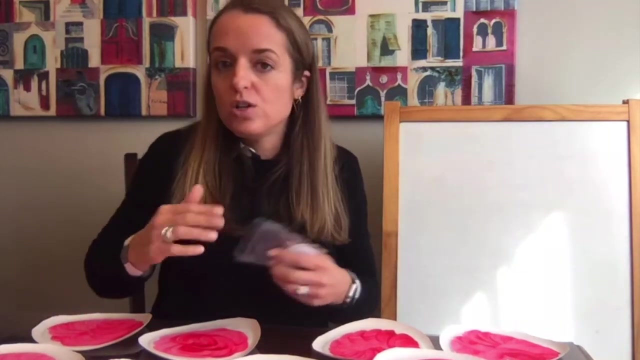 found some pictures, printed them, laminated them and cut them out Again. I'm going to be saving these um for three years because you'll use these again, Easy peasy, Okay. So give the kids all of these ingredients and tell them: make a pizza. make it, however you want. Um you can use. 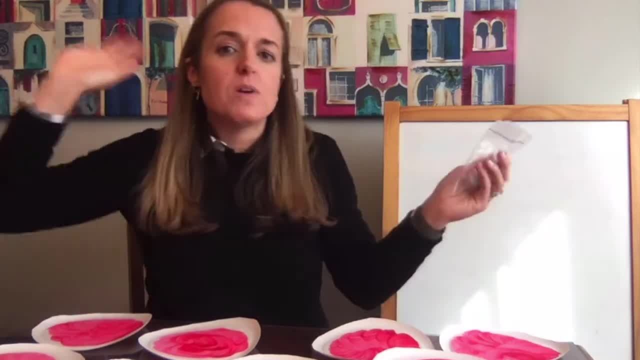 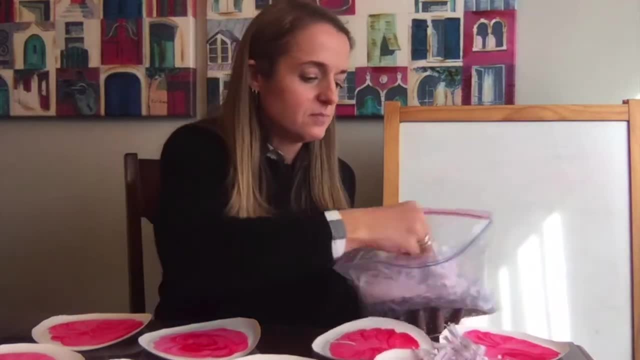 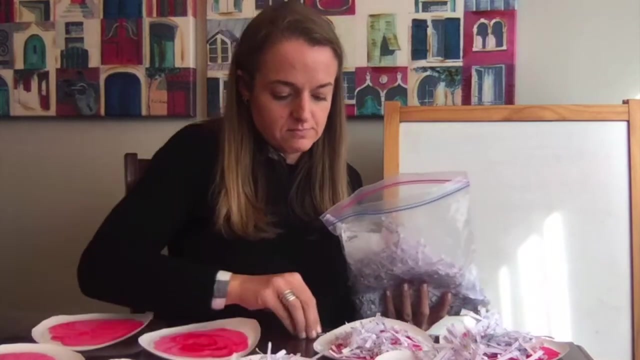 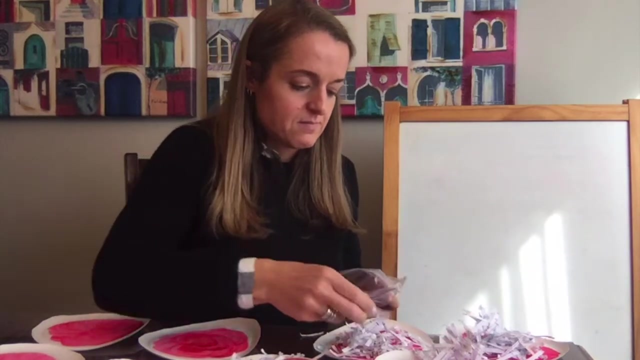 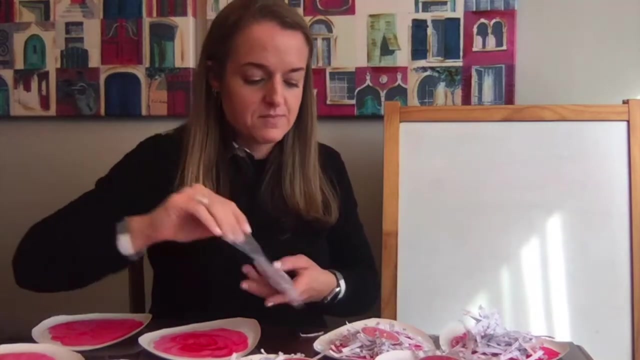 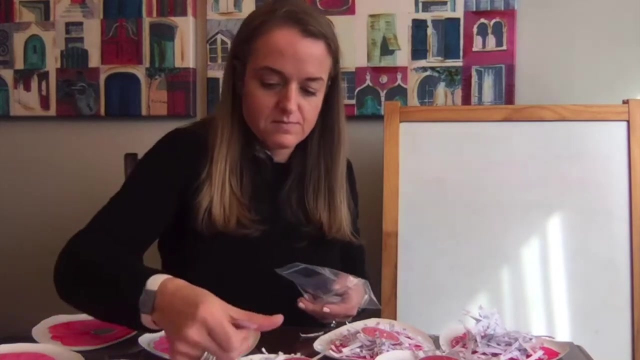 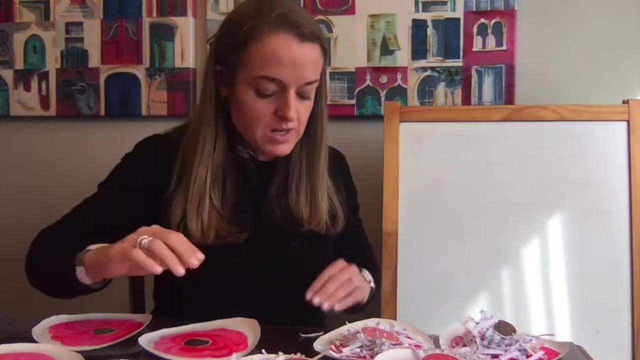 all the ingredients. You can use none of the ingredients. You can use one, two, three. just make your pizzas. Okay, So I'm going to make my pizzas. now I'm going to try and make them different. Okay So, I used my three ingredients and now let's see which pizzas I made. So now we want to go to 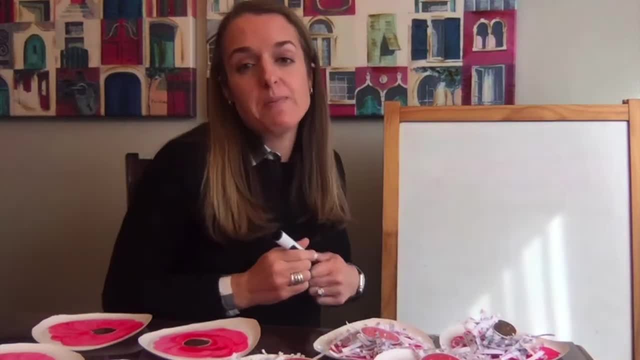 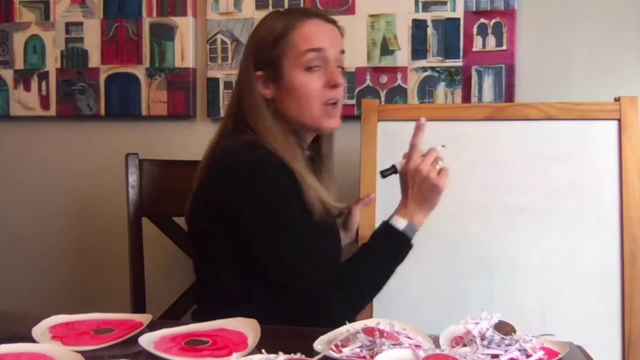 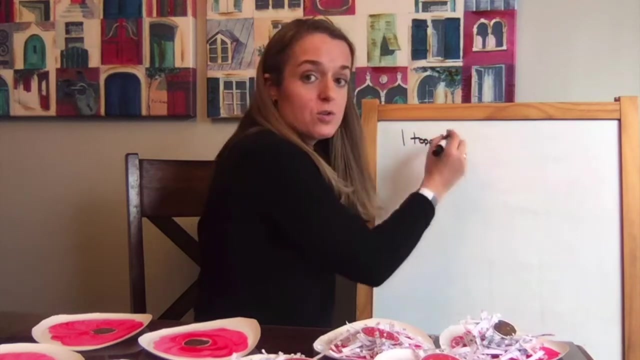 the board and the kids can have a piece of paper themselves and make a chart also. Okay, We want to just list the pizzas that we made. So we're going to have three columns, We're going to have one topping pizzas and what those choices are. 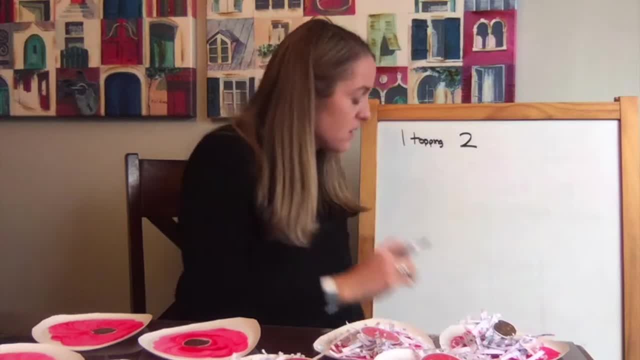 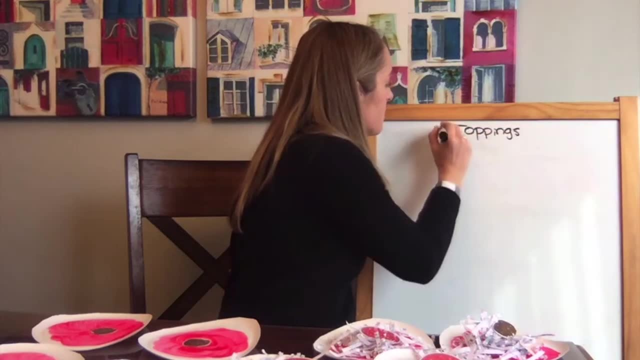 and we'll write it out. We're going to have two topping pizzas. Hang on, I'm going to do this a little different. All right, so toppings are going to be on the top. okay, The number of toppings. So we're going to have one. sorry guys not liking my charts. 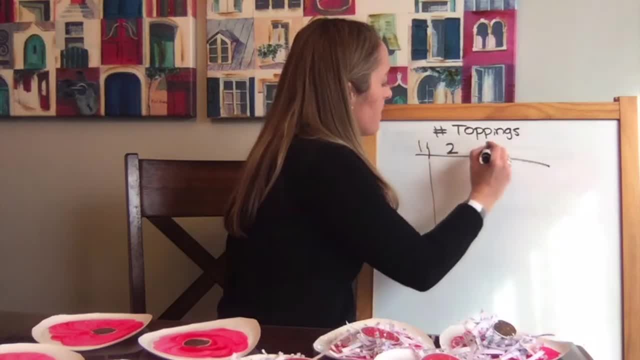 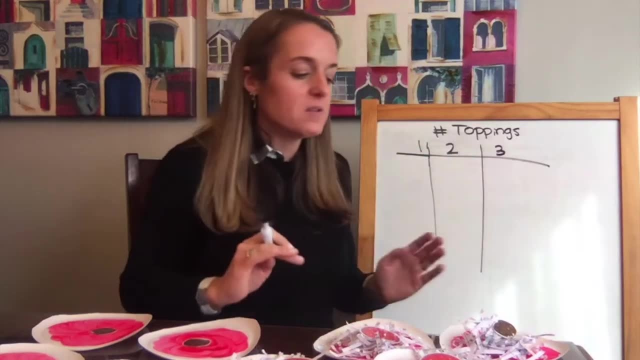 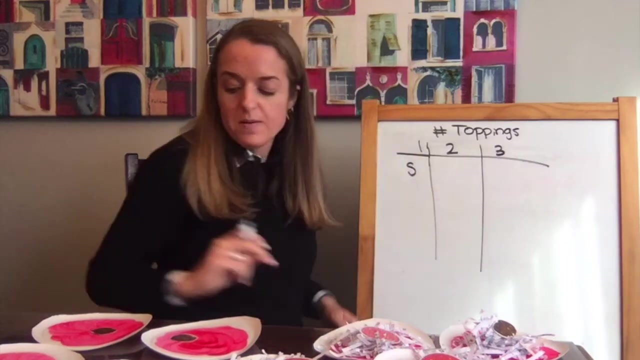 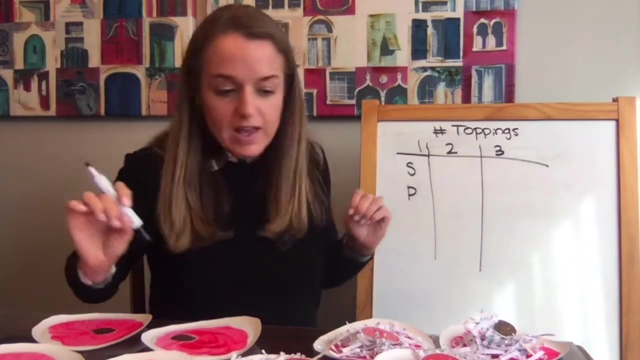 There we go. One topping, two toppings, three toppings, Okay, so what one topping pizzas do you see that I have? I've got a sausage pizza, so I'm going to just do S for sausage. okay, I've got a pepperoni pizza and that looks like my only one. to other one topping. 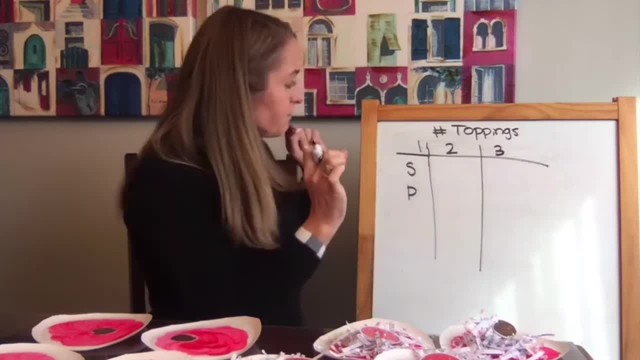 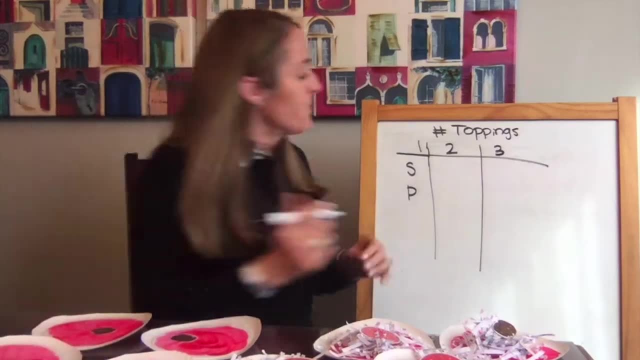 pizzas. We may be missing some, but we'll figure it out in a minute, okay, What two topping pizzas do I have? I see pepperoni and sausage. So I'm going to say pepperoni, sausage. I see cheese and sausage. 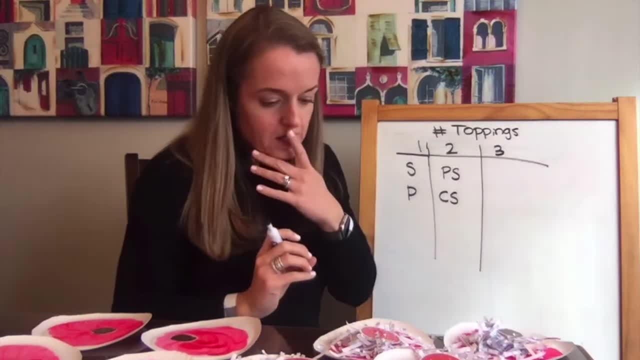 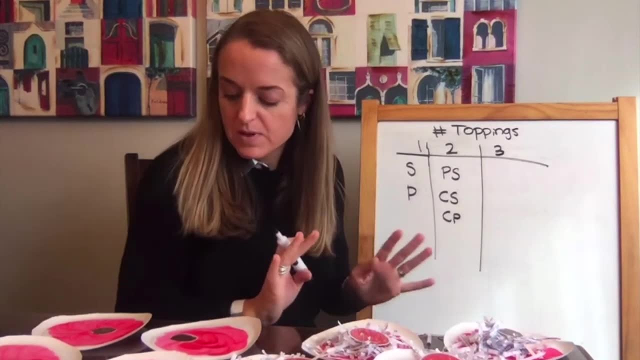 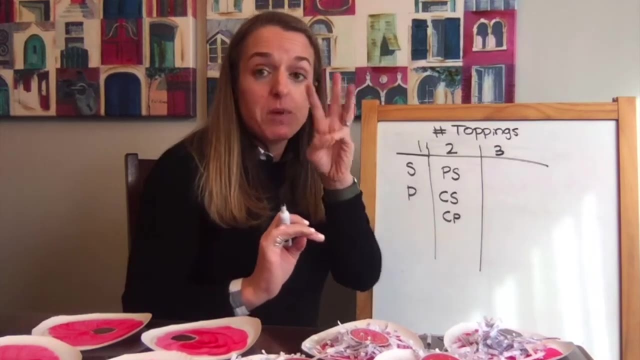 I see another two topping. Oh, I see cheese and pepperoni. Okay, I don't see the other two topping pizzas. Cheese and sausage- I got that- and cheese and pepperoni. Okay, how about three topping pizzas? I see cheese, pepperoni and mushroom. 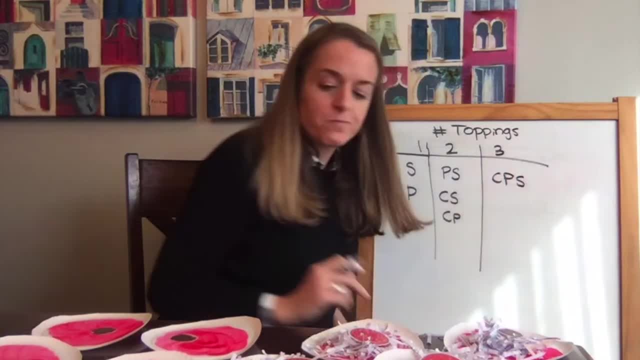 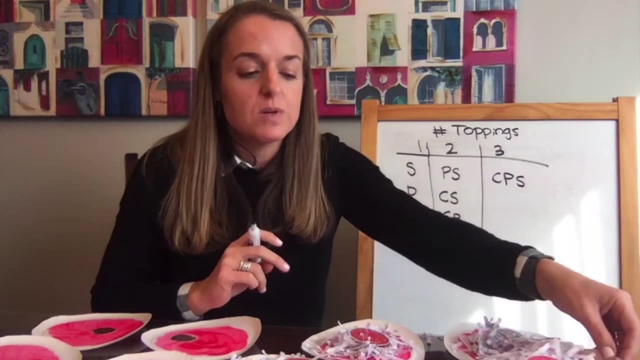 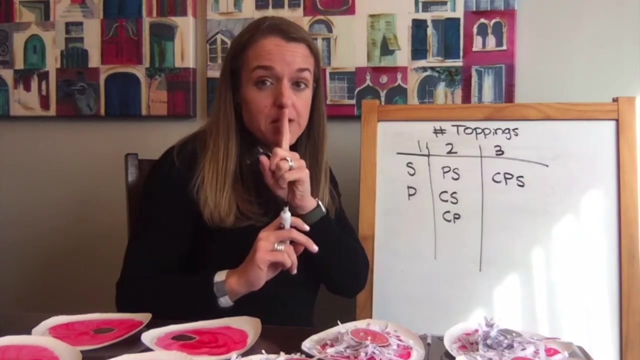 I'm sorry, cheese, pepperoni and sausage. I've got two of those. Looks like that's my only three topping pizza And adults. it's really handy to have a cheat sheet just as a note, because we are we're missing one kind of pizza. We are missing a one topping. 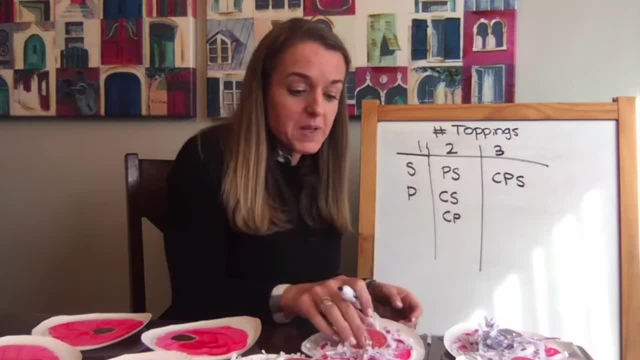 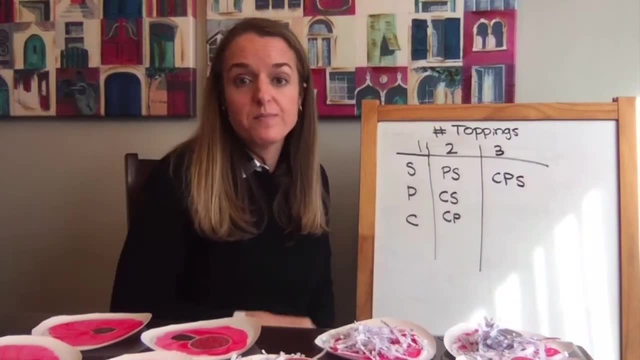 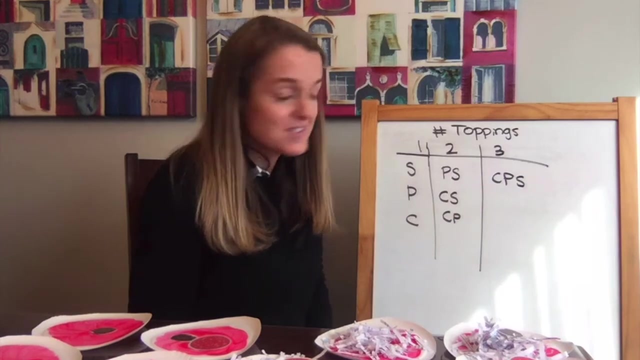 pizza. What did I not make? I didn't make a cheese pizza. Check it out: There's a cheese pizza, Plain cheese pizza. So how many different pizzas did we make? did we make here One, two, three, four, five, six, seven? We made seven pizzas when we had. 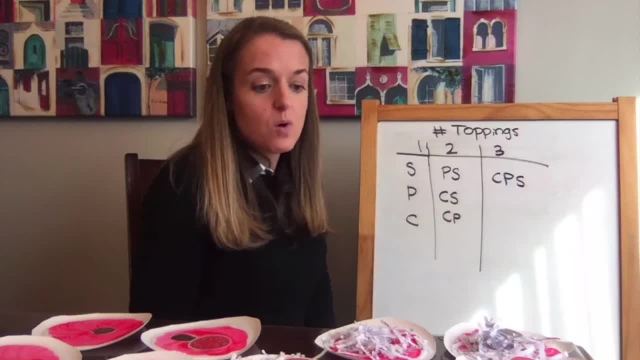 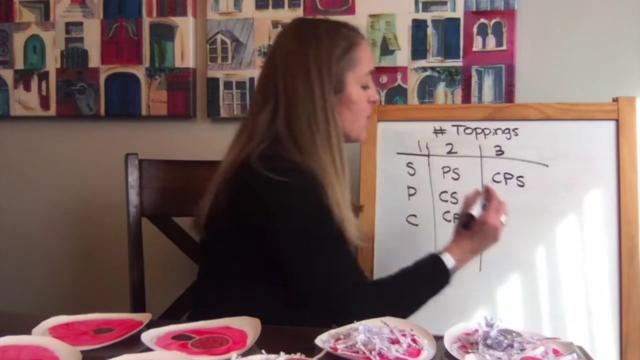 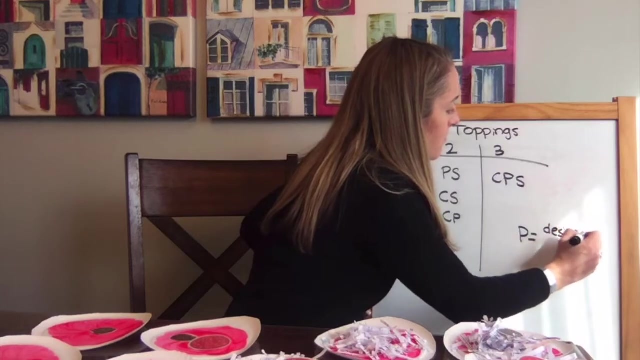 three different toppings. So, um, there are seven possibilities. So the probability of getting the one you ordered, if you order a cheese pizza, the probability that you will get a cheese pizza. So remember that our equation is: probability is desired outcome over the total right The total. 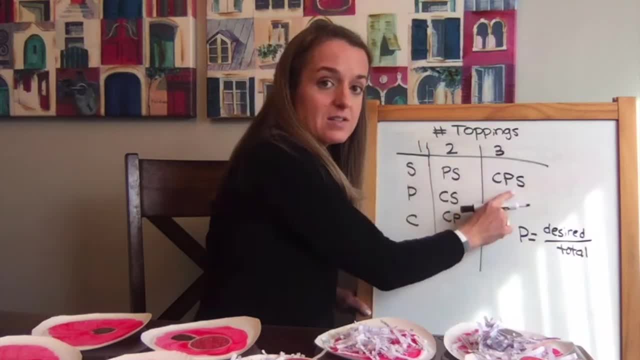 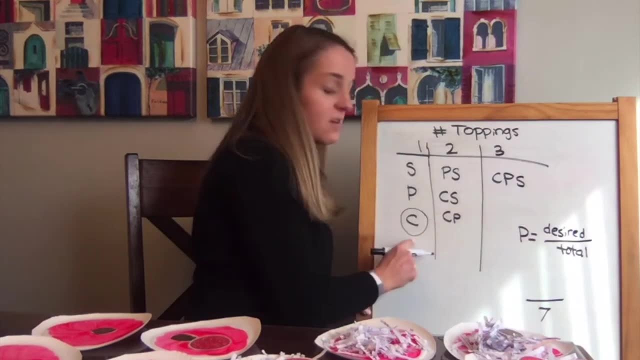 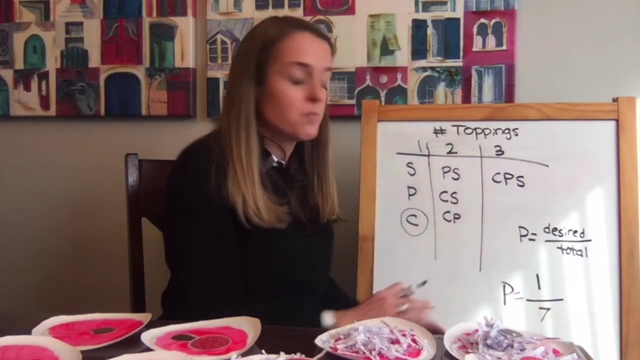 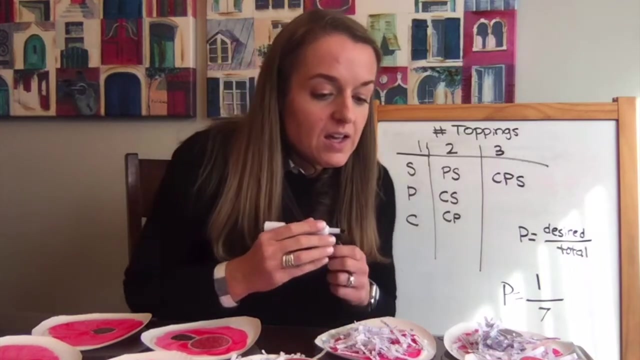 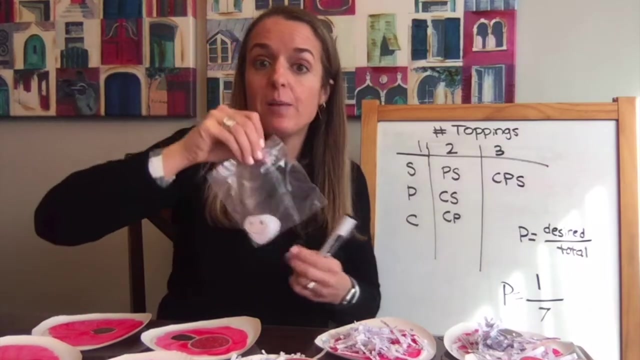 outcomes. So here we have seven pizzas. So seven is how many total outcomes there are, And our desired outcome is for a cheese pizza. So that's one pizza. So our probability is one over seven. That is our probability of getting The pizza that we want. What if we add another topping? We add mushrooms, How many different? 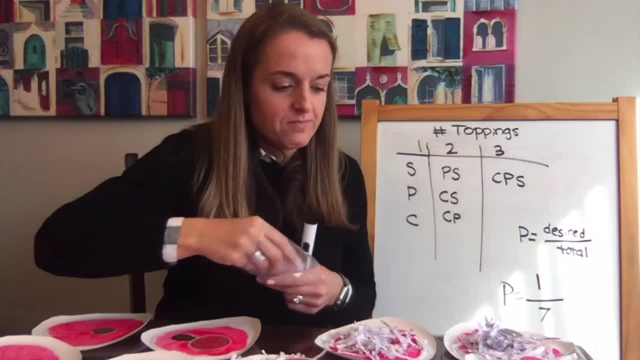 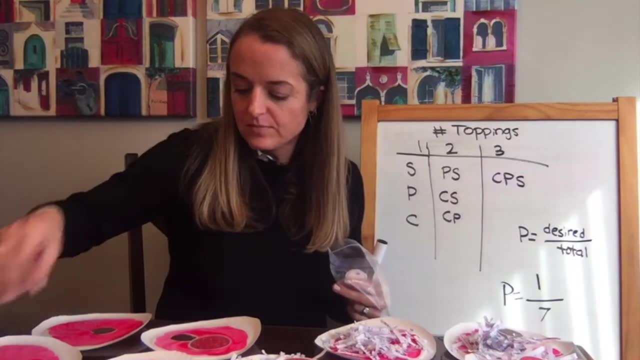 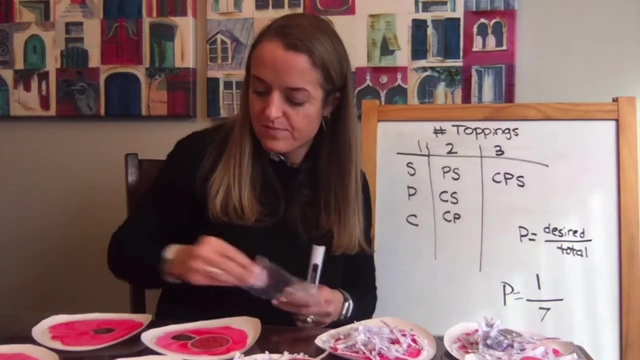 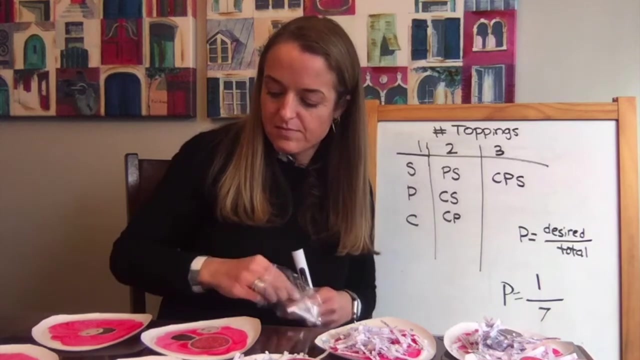 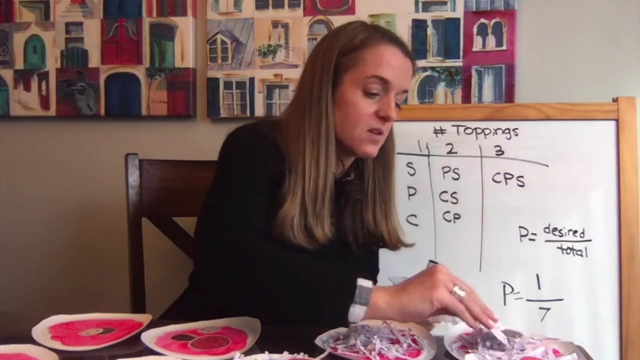 pizzas can we make now? So let's see, let's try and eliminate our duplicates here. That one was a duplicate. Oh yeah, We're going to need some more pizzas, aren't we? We're going to need some more pizzas to show what's. 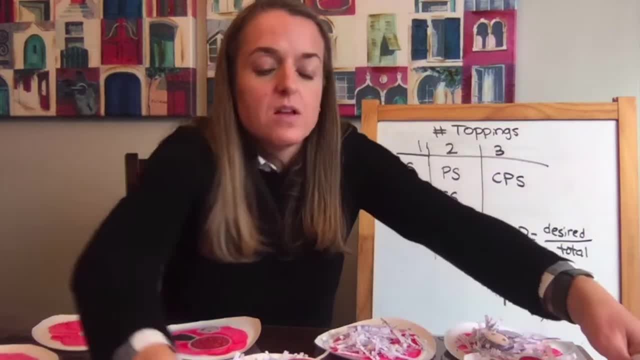 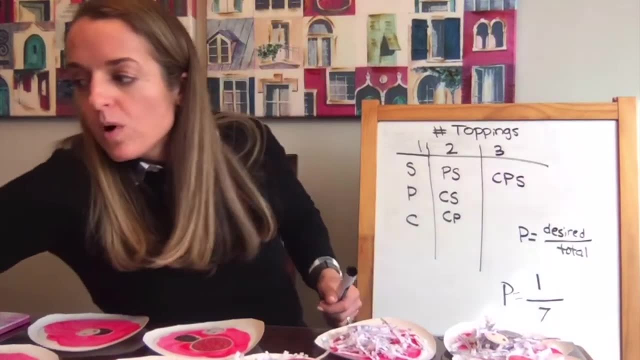 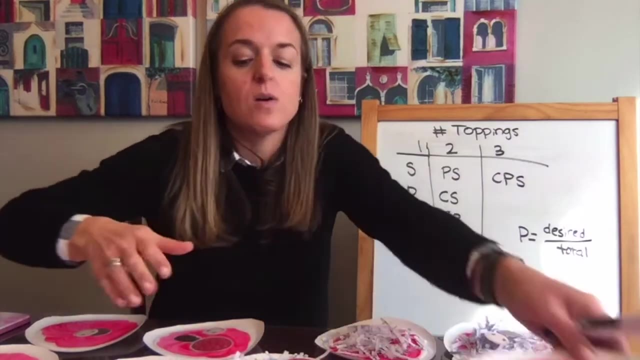 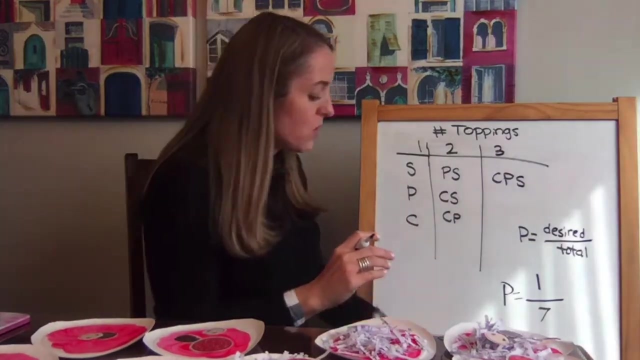 going on. So you guys can keep making, can keep doing more pizzas. I have more pizzas over here. We can keep making them and see if we can make more pizzas. So, as the kids are making them, we can then, after they're done making the different kinds of pizzas we can add to our list. So what pizzas have we made now? 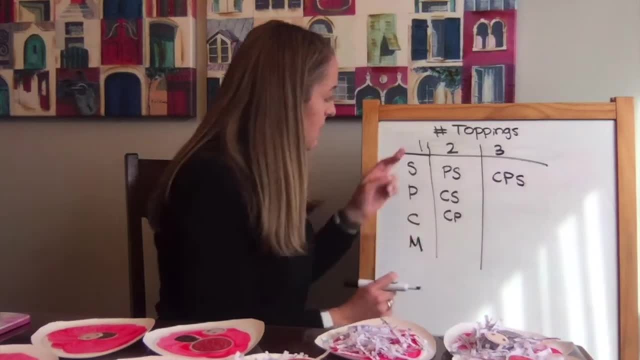 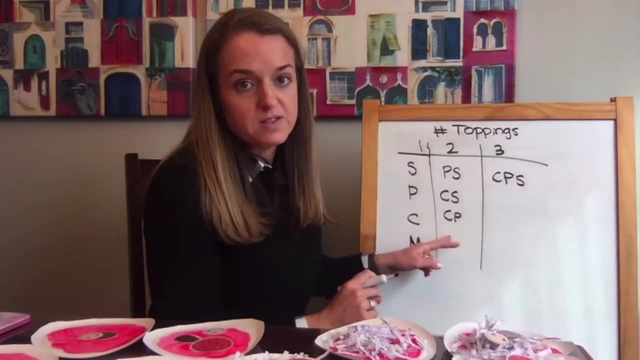 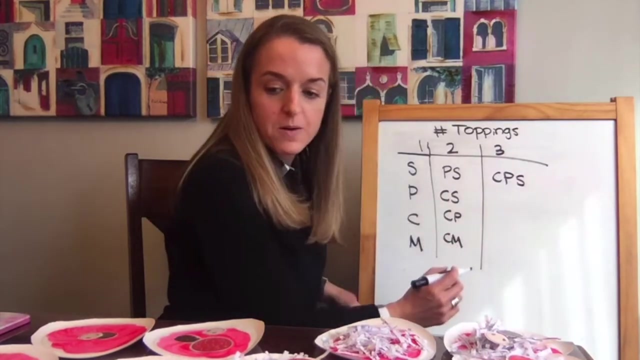 We have now made a plain mushroom pizza as our one topping pizza. That's our only additional one topping pizza. How about two topping pizzas? What additional two topping pizzas have we made? So we still have these, but adding mushrooms. we were able to add cheese and mushroom, pepperoni and mushroom sausage, and mushroom. And then what about three topping pizzas? We add cheese, pepperoni and mushroom, cheese sausage and mushroom, pepperoni, sausage and mushroom. And that is all for the three topping pizzas. but did somebody make a four topping pizza? I have it right here. So we have a new column for four topping pizzas. We have one four topping pizza cheese, pepperoni, sausage, mushroom. So we've done four toppings now. but what would happen if we then added a second crust size? So we call this regular crust.